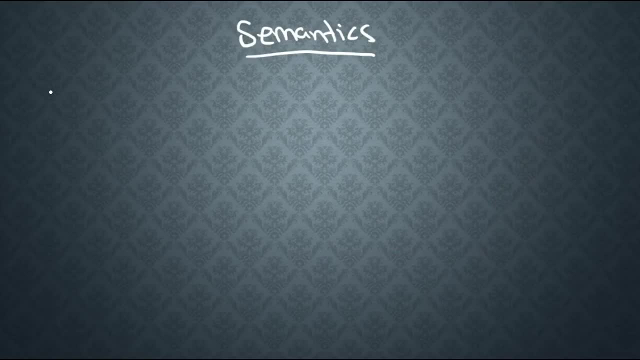 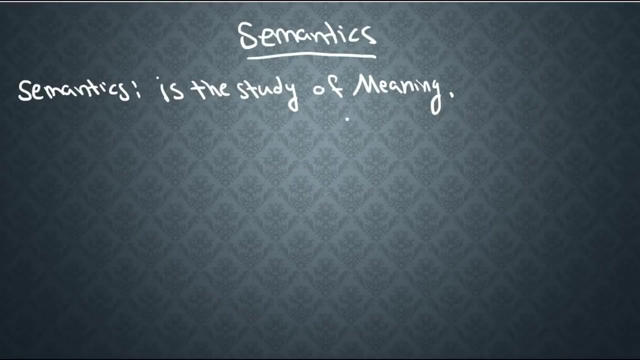 Email me at any time. So let's begin. What do you think semantics is? Well, let me help you out with a starter definition. Let's say that semantics is the study of meaning. So here's what I want to ask you guys: What type of meaning are we looking at here? Well, it could be meaning that we find in life. It could be meaning that you find in a painting. 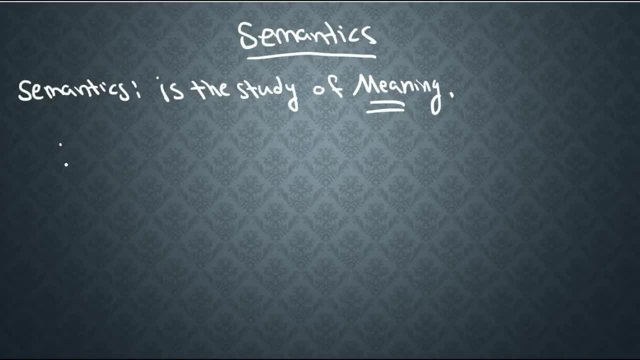 It could also be meaning that you find in music. However, the meaning we are concerned with here is the meaning you actually find in language. So let's fix up our definition just a little bit. So semantics is a study of meaning and language, but we're still not done here. What type of language are we talking about? Is it Are we actually studying meaning in Spanish, in English, in Arabic? Well, the fact of the matter is, if we're going to study meaning in each and every one of them, 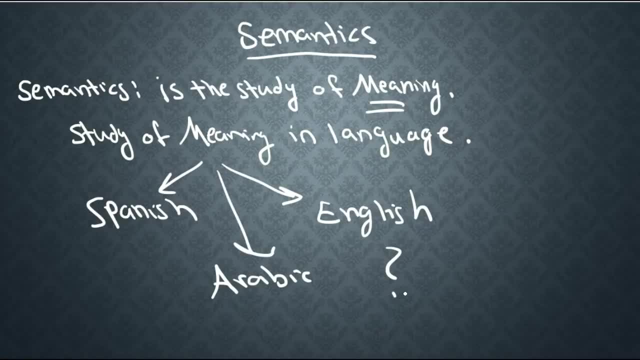 one of these languages individually. this is going to take us forever And we probably won't come up with the generalizations that we're looking for. So it is very important to make a distinction between language and language. Language with a small L and language with a big O. Language with a small L is just a name we use to identify the languages we use on a daily basis Again, like English, Arabic and so on and so forth. 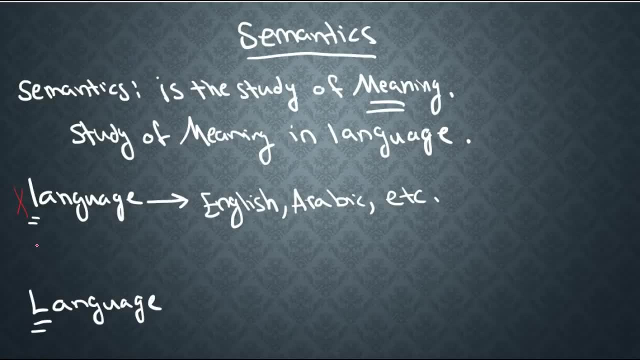 Now we said: this is not the type of language we want. So we're actually interested in language with a big L. So whenever we use this word, language with a big L- what we're actually looking for or what actually means, is the principles of human language, And I use LG as short for language. We could also be dealing with the algorithms of human language. For now, you can call it whatever you want. 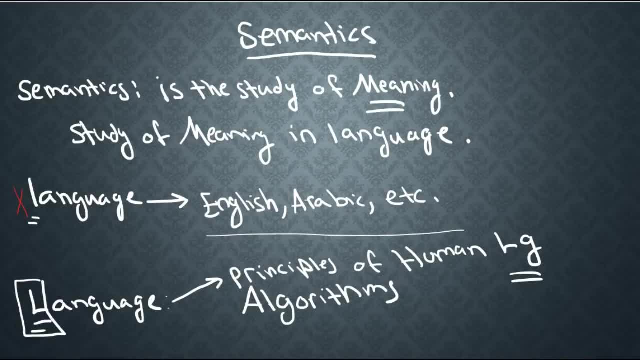 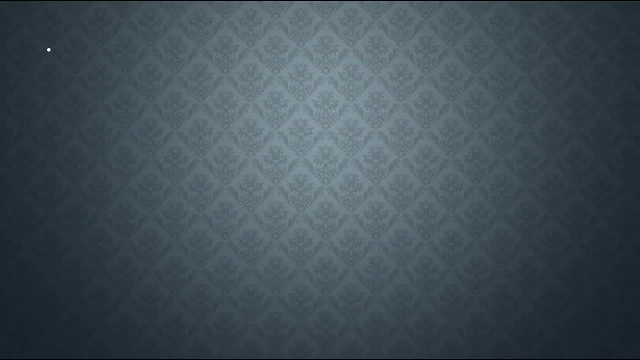 Really it's just you know what makes up human language in general. So we're looking at universal terms here, not language specific. So now let's try to formalize our definition a bit better. So semantics is the study of meaning in human language. Meaning in human language. 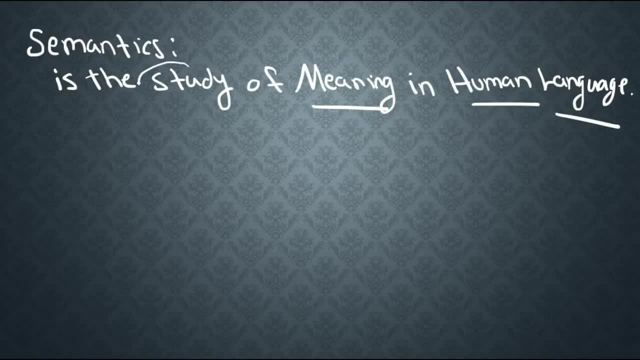 There's one more content word let's say that we've left out, And that's study. What do we mean here By study? How is this a study? What branch of science is semantics a part of? So, when we talk about semantics as a study, what we're really talking about is that it's part of the study of linguistics. Now, linguistics is the study of human languages, And actually this should be a big L. So let's start with a little example: Lily ate the apple. 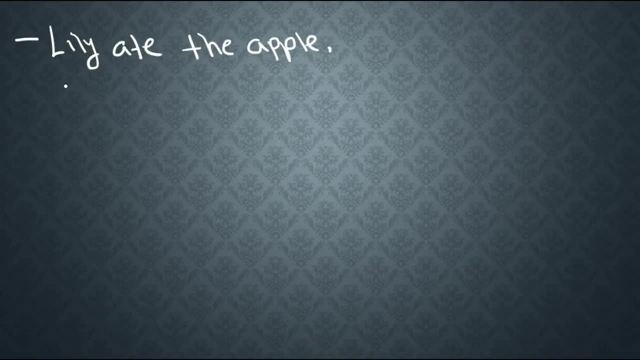 What is this sentence made of? So, what is this sentence made out of? Well, as you can see, it's made out of words like Lily ate the apple. These words are built together to make up phrases, for example, like this noun phrase right here. Okay, But going on to a little smaller level, we have sounds. So L is a sound, I is a sound, Right, T is a sound, H is a sound. So all of these are made up. 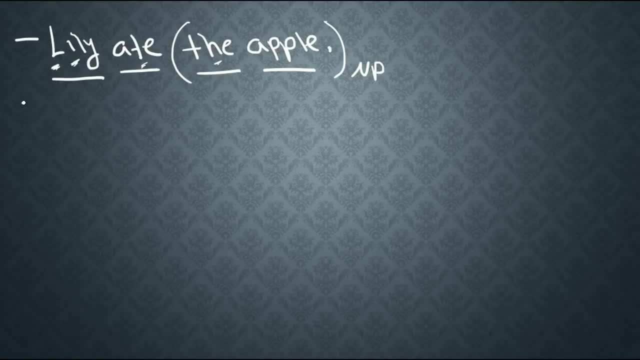 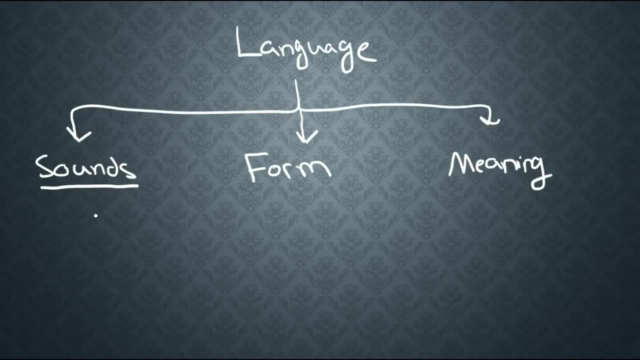 These components combine together to create language. So let's take a look at exactly how that happens. So language is divided up into three basic components, The first of which is sounds, The second part, you could imagine, is form And the third part is meaning. So now, under sounds, we're actually dealing with the individual sounds of the language. like we mentioned, the L 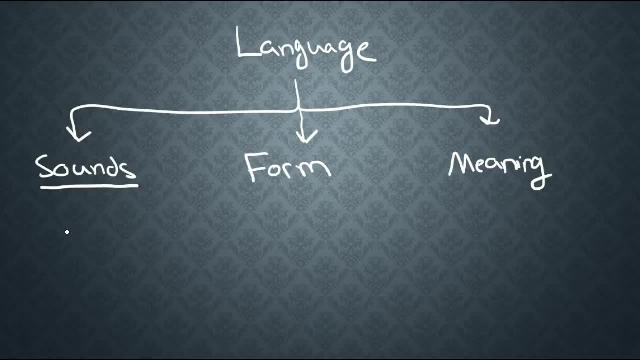 Sound in Lily, The sound in the word the Okay And the sound in the word apple. So the branch of linguistics that studies sounds is called phonetics. There's also one more branch called phonology, which is closely related, but that's kind of out of the topic right now. Next we have form. Now, after we have these sounds, we need to form them up. 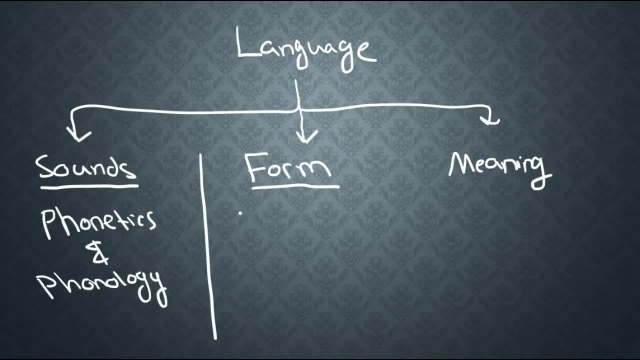 In a certain way, Right? So first we need to make words out of them, And then we need to make these words combined together to form phrases. Okay, So what we're looking for here is words, And then we're also looking for phrases, And these phrases actually combine together to give us clauses, which are basically sentences. Okay, So the part of linguistics that studies words is called phonetics. 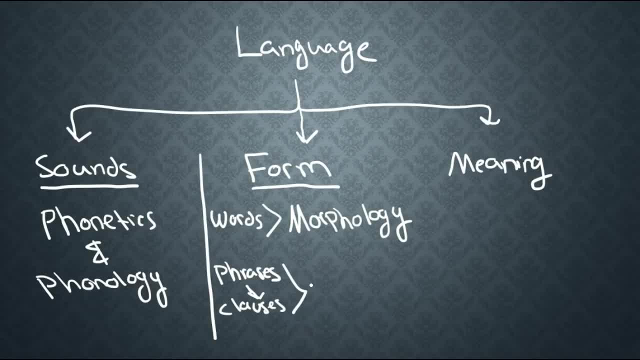 Morphology, And the part that studies phrases and clauses is called syntax. Now we move on to the part that interests us in this course, which is meaning. Now, meaning can come about basically on the sentence level, or it can come about above the sentence level. So meaning is basically studied by two branches of linguistics, The first of which is semantics And the second of which is pragmatics. 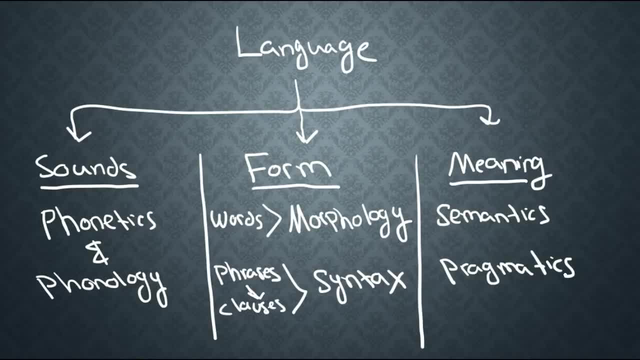 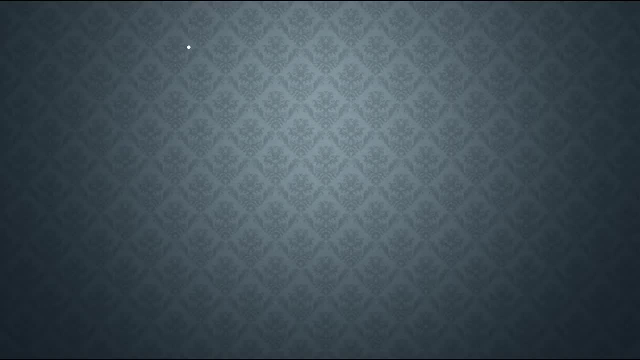 Now, this list does not in any way cover all of the sub branches of linguistics, but it'll do. for now. We talked about the language components. Now, what is a grammar of a language? Well, grammar here is certainly not the type of grammar you took at school. So grammar does not mean that we're going to talk about if statements or present progressive 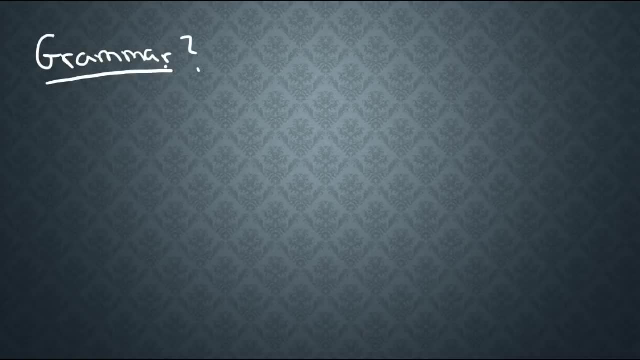 Right. Actually, what we are looking for here when we say the word grammar is every single part of a language, every part that you need to make that language work. So, basically, you're talking about the sounds, right. You're talking about the syllables, Also morphemes. You're also looking at the words that arrive after you say the word. 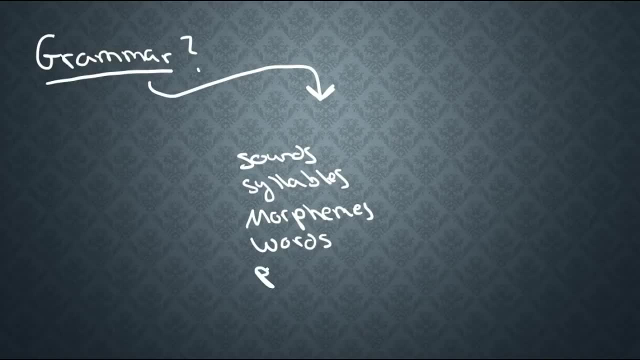 Or you know, connecting your morphemes, And then you're looking at your phrases and your clauses and sentences, Right? So within this grammar, we said, of course, that something like sounds and syllables will be studied by phonetics and phonology.